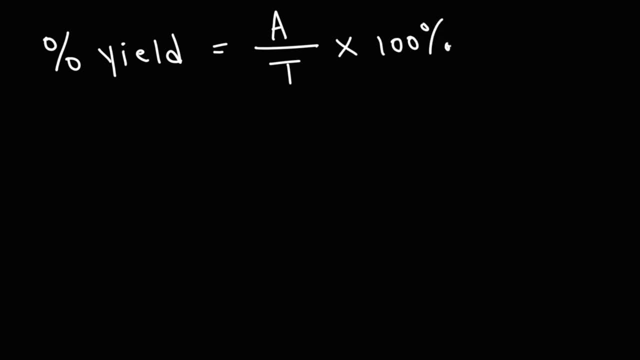 it by the theoretical yield and then multiply that by 100%. I do have a video that explains how to calculate the percent yield. For those of you who want some practice problems on that, feel free to check out the links in the description section below. Now, sometimes you may need to calculate percent yield, but you don't. 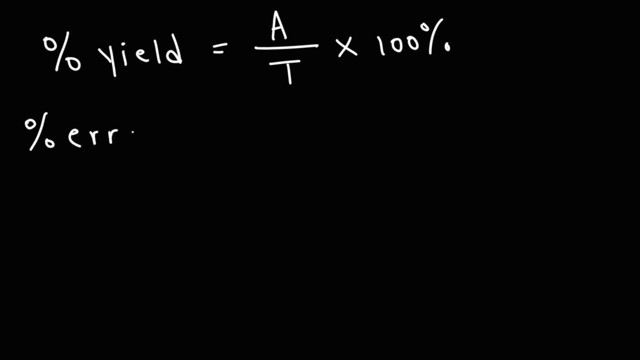 necessarily have to. So I'm going to show you how to calculate the percent yield. For those of you who want some practice problems on that, feel free to check out the links in the description section below So you can calculate the percent yield. 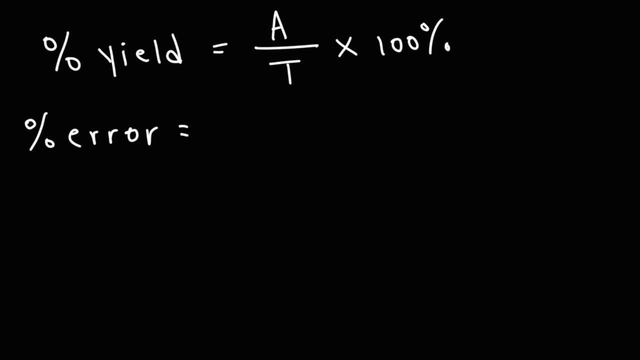 This is not as common as percent yield in a typical chemistry class, but if you do need to calculate it, here's the formula: Percent error is actual minus the theoretical, But it's really the absolute value of that difference. So whether you subtract A by T or T by A, you're still going to get a positive. 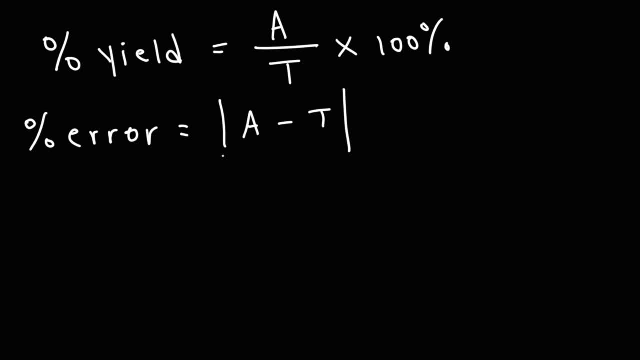 result if you place it within the absolute value symbol. So it's the actual yield minus the theoretical yield. So it's the actual yield minus the theoretical yield Divided by The theoretical yield times 100%. So that's how you can calculate percent error. 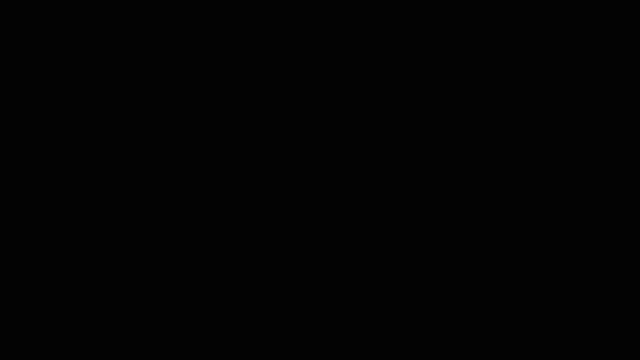 Now, when dealing with percent composition problems, you need to know how to calculate the mass percent of an element. The mass percent of an element, The mass percent of an element, is going to be the mass of that element divided by the total mass of the compound, multiplied by 100%. 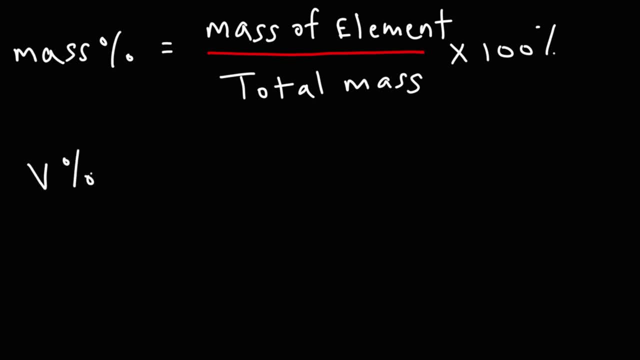 So that's mass percent. It's also something known as volume percent. It's going to be the volume percent. It's going to be the volume percent. It's going to be the volume of the element or substance divided by the total volume times. 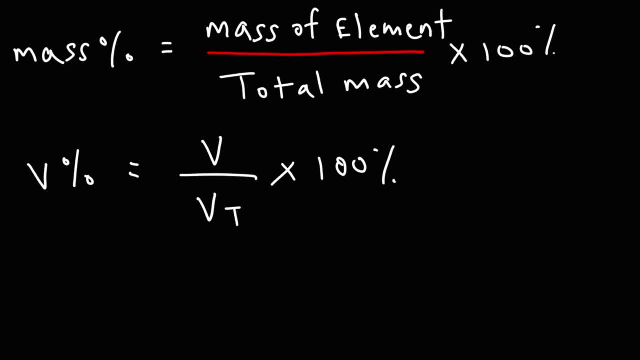 100%. So that's how you can calculate mass percent and, if needed, volume percent. The mass percent formula is going to be very useful when dealing with problems such as empirical formula determination. You know that's where you'll typically use it as well. 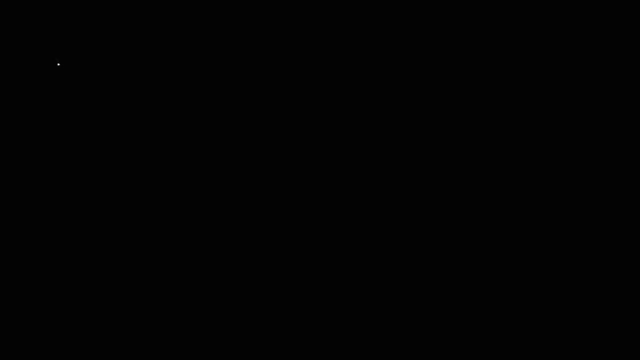 Now for those of you who are studying solutions stoichiometry, you need to know how to calculate the concentration. The concentration is going to be equal to the moles divided by the volume. Now there are different forms of concentration out there, but the first one that you most 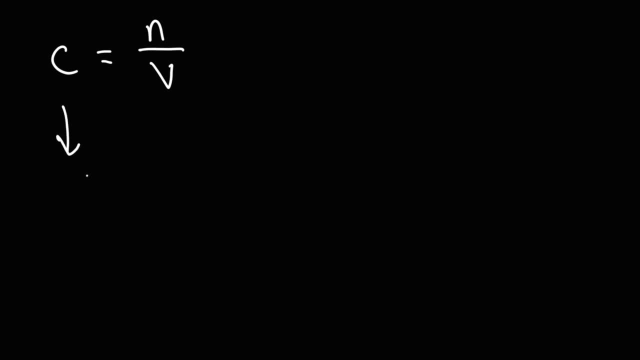 likely encounter is molarity. So this concentration is molarity. You can write this formula as capital. M is equal to N over V. It's equal to the number of moles divided by the volume in liters. Now remember, one liter is 1,000 milliliters. 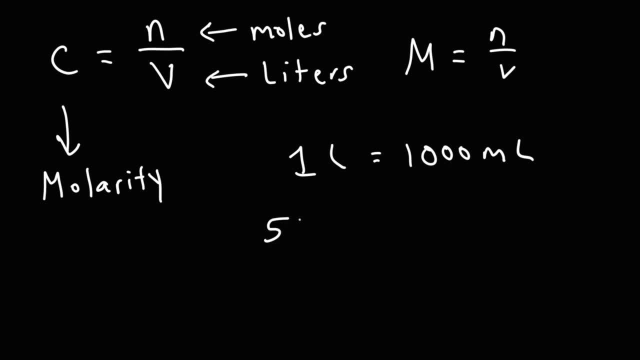 So if you're given the volume in milliliters, let's say if you have 540 milliliters to convert that to liters, simply divide by 1,000. And this would be 0.54 liters. Okay, Also, one kilogram is 1,000 grams and one gram is 1,000 milligrams. 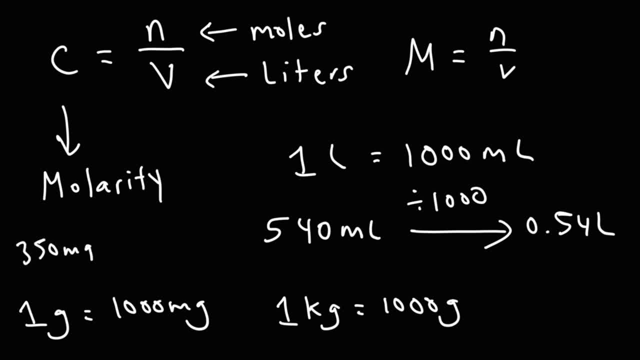 So in the event that you're given the mass in milligrams and you need to convert it to grams, divide by 1,000.. 350 milligrams is 0.35 grams, But whenever you need to calculate the molarity, it's moles over volume. 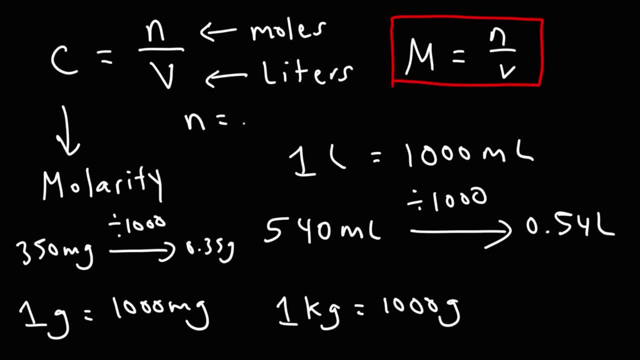 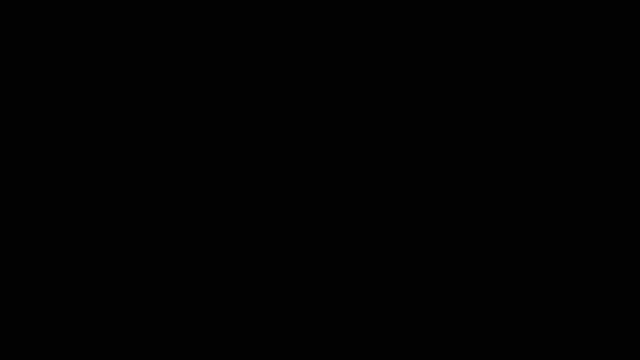 If you need to calculate the moles, it's going to be the molarity times the volume. Now, when dealing with dilution problems, this formula will be useful: M1 V1 is equal to M2 V2.. And we know that the molarity times volume is the moles. 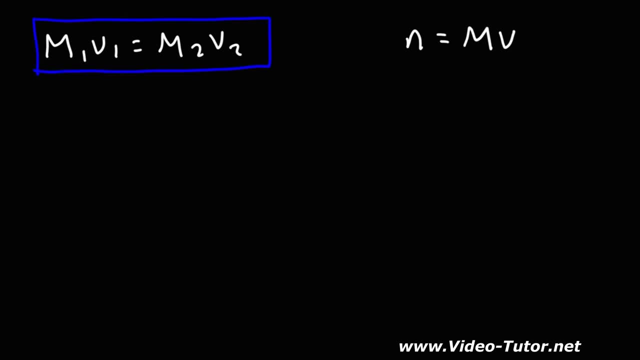 So let's say, if you have a solution and you add water to it, The volume is increasing, but the moles of substance or solute in that solution stays the same. So that's why these two can equal each other. But as the volume of the solution goes up, the concentration of that solute goes down.